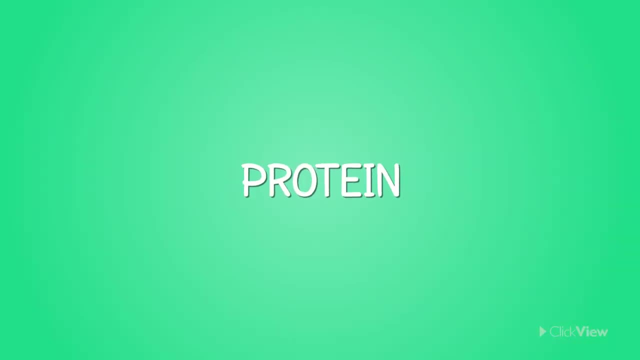 the day: Protein. It is very important to include foods rich in proteins in our diets every day, as they are important for the growth and repair of our bodies. Protein-rich food to include in our diet are lean meats, eggs, fish, tofu and vegetables. Protein-rich foods are rich in. 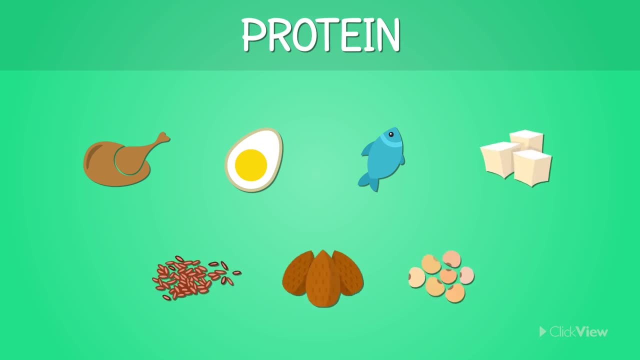 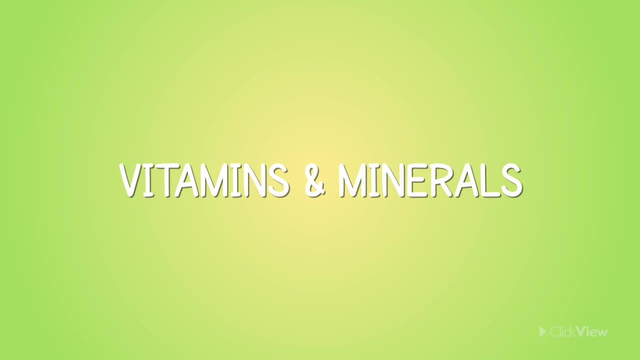 protein, vegetables, vegetables, vegetables, vegetables, vegetables, vegetables, seeds, nuts and beans. Vitamins and minerals. Vitamins and minerals are essential to keep us healthy. Did you know that they help us grow, help us to see, keep our organs, bones, muscles and skin healthy? 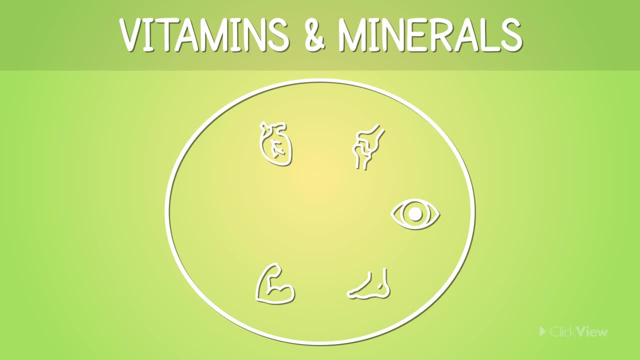 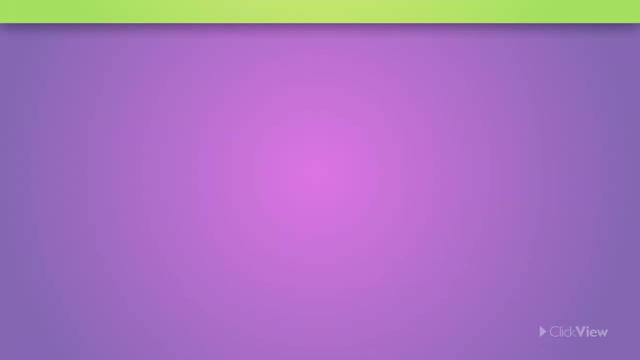 as well as help us to fight diseases. Vitamins and minerals can be found in all types of fresh fruits and vegetables, vegetables, fruits, vegetables, vegetables, vegetables, vegetables, vegetables. Calcium: Calcium is an incredibly important mineral. Calcium is stored in our teeth. 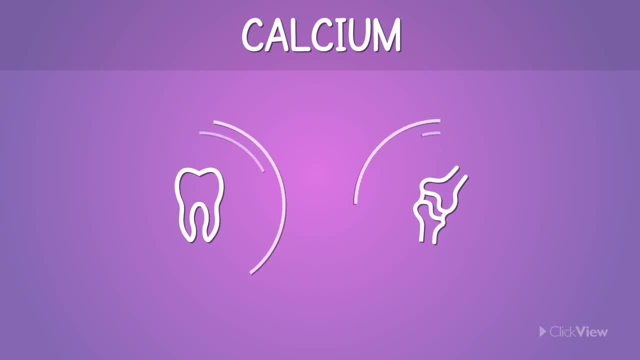 and bones and keeps them strong and prevents cracks and breaks. You can find calcium in dairy products such as milk, yogurt and cheese, as well as leafy green vegetables, nuts and seeds. Fibre. Fibre is a very important mineral in our diet. It is a very important mineral in our diet. 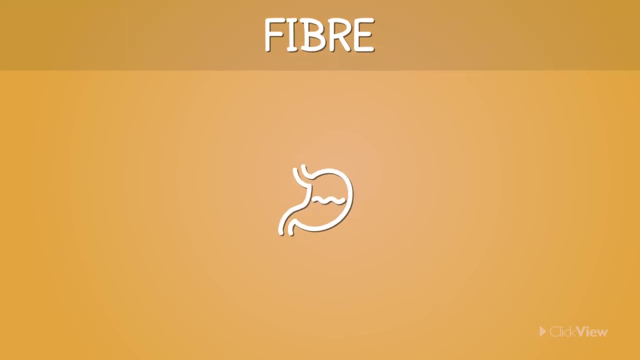 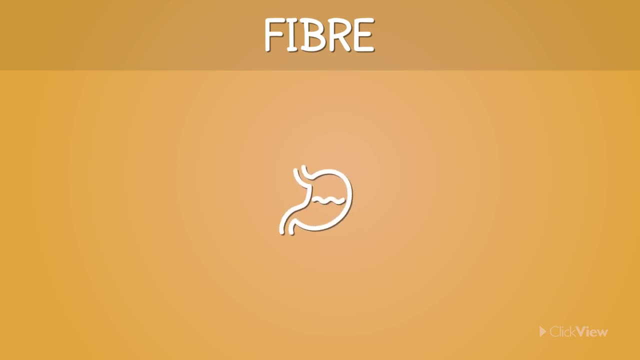 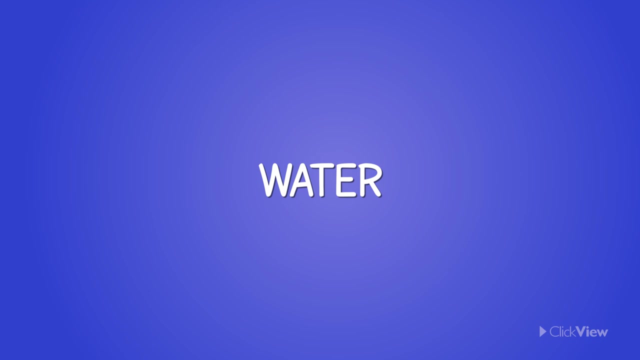 bodies and stay healthy. Fibre can be found in foods such as brown rice, whole-grain bread, cereals, nuts, seeds, fruits and vegetables, Water. Water is essential for helping your body digest and use the nutrients bound in the foods you eat every day. 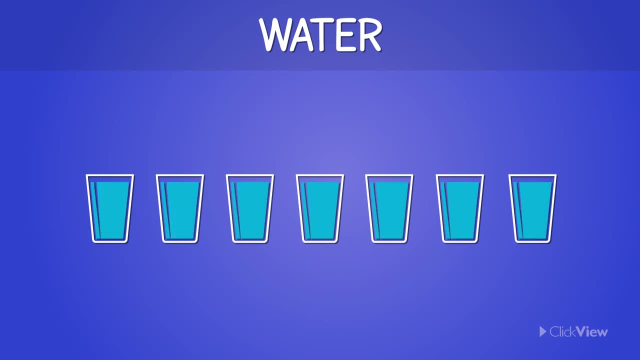 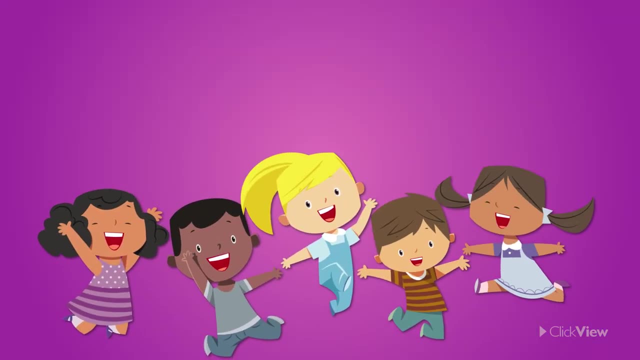 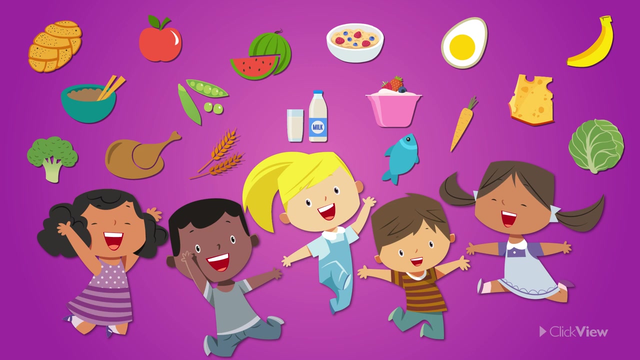 Therefore, it is important to drink lots of water every day to help with this process. It is very important to ensure that your daily diet includes a variety of all these foods. Having a balanced diet makes sure that our bodies receive all the nutrients we need.